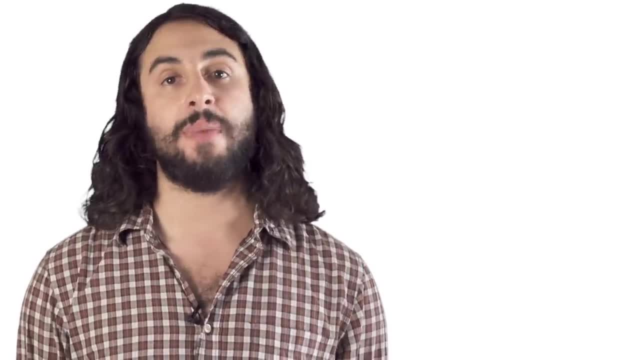 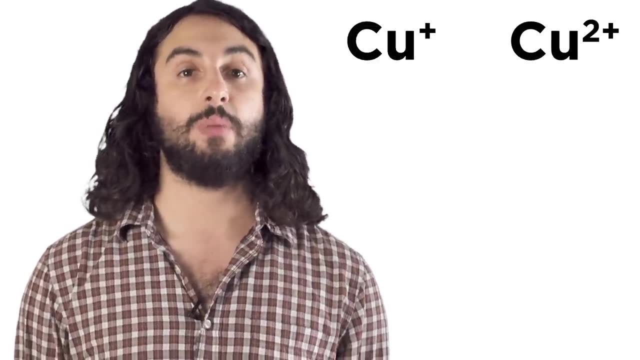 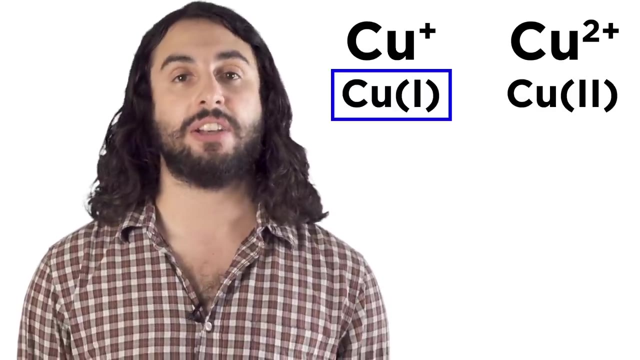 That makes this sodium chloride. Some metals can have different common charges or oxidation states. Copper can be one plus or two plus, and we represent that with roman numerals in parentheses. Copper one means that it is a one plus ion and copper two means two plus. 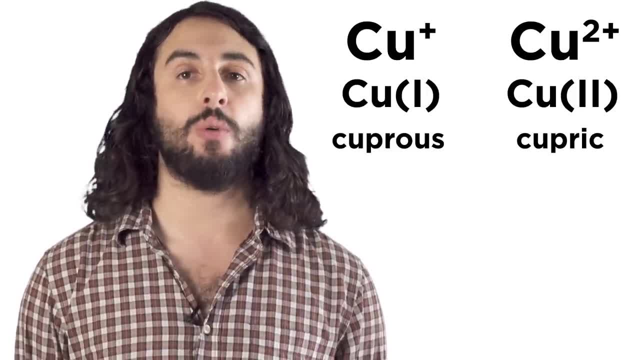 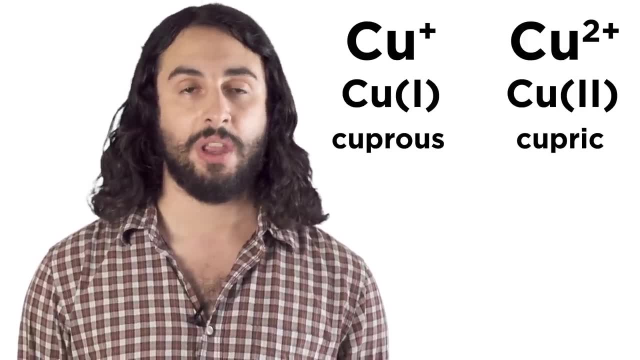 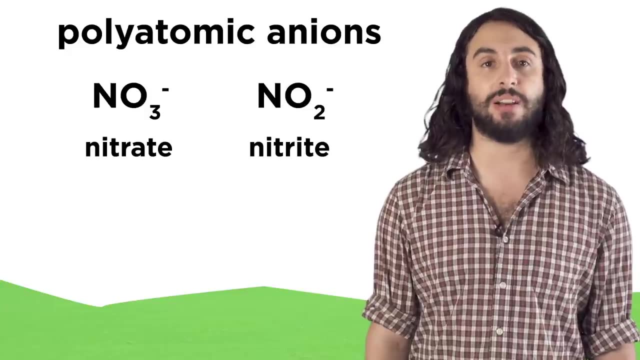 If there is an element with two common oxidation states, the lower one bears the suffix "-us" and the higher will be "-ic". So a copper one ion is a cuprous ion and copper two is a cupric ion For similar polyatomic anions with different numbers of oxygen atoms in them. 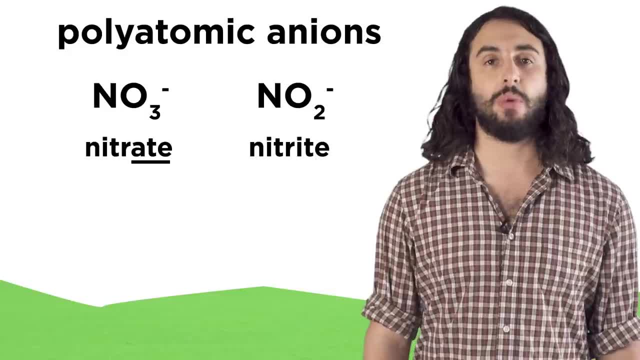 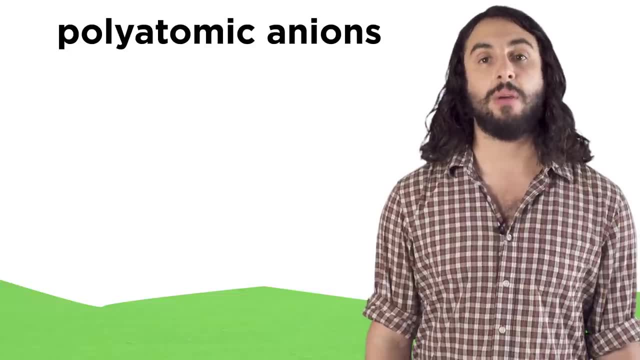 the one with more bears the suffix "-ate", The one with less bears the suffix "-ite". So this is the nitrate ion, and this is the nitrite ion. If there are more still, we can use the prefixes "-per-" and "-hypo-". 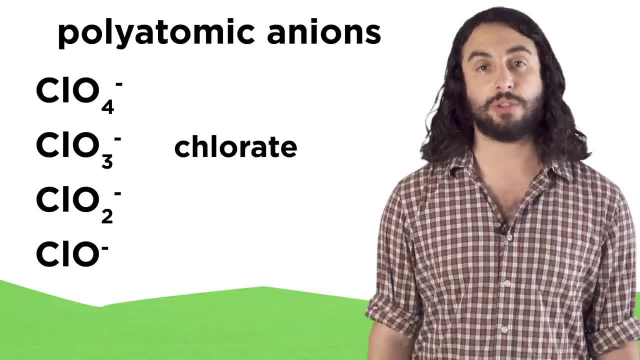 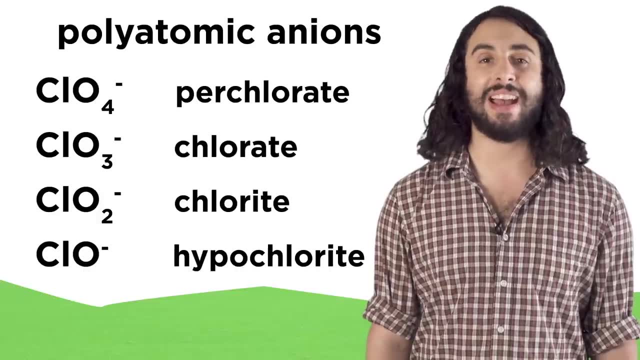 in addition to the suffixes. So this is chlorate, this is chlorite, this is hypochlorite and this is perchlorate. These prefixes and suffixes are used as necessary, depending on how many variations a particular ion has. 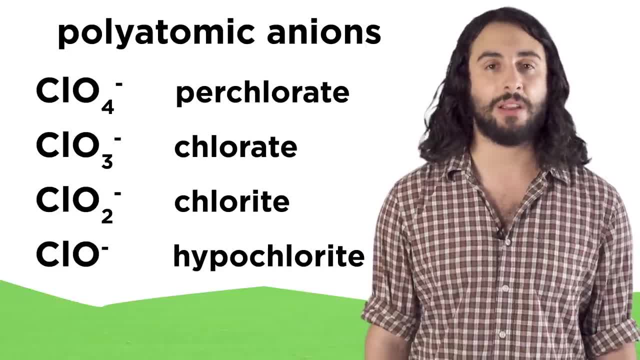 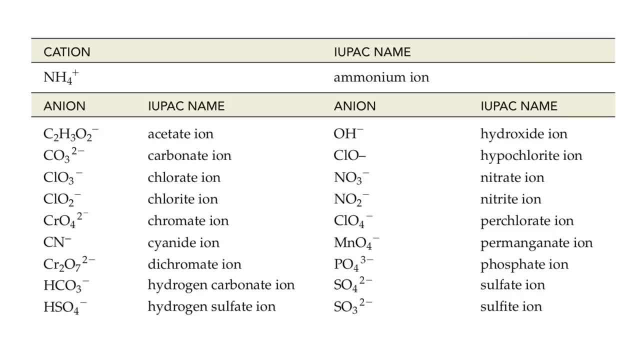 There's not very much memorization in chemistry if you understand what's happening, but unfortunately, knowing the names and charges of these polyatomic ions is a case where you're just going to have to memorize a little. These are the most important ones to know by name and their charge. 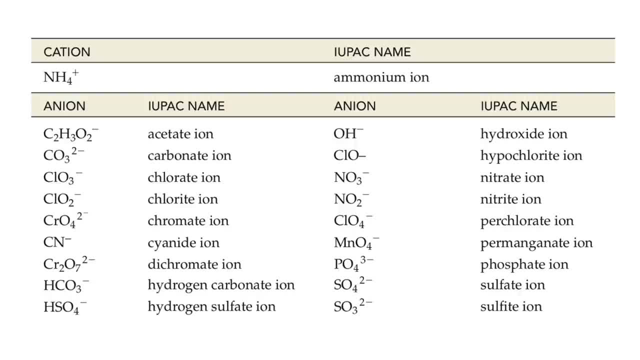 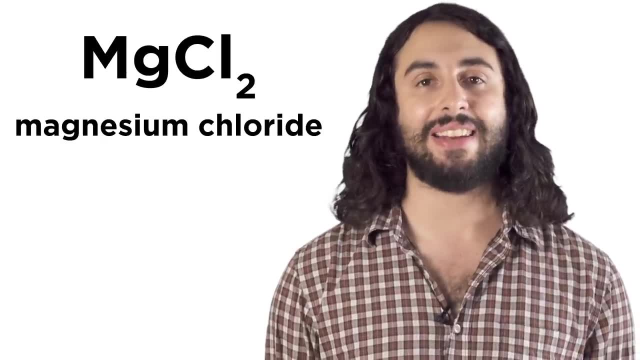 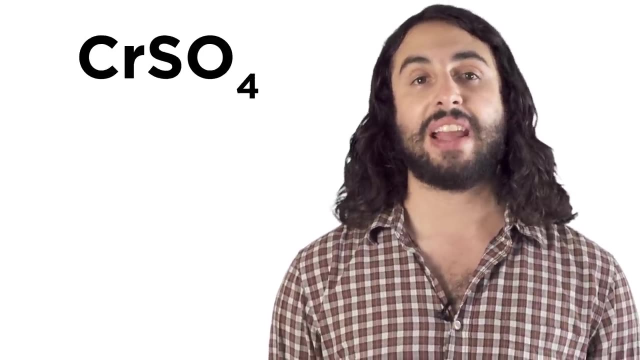 Putting it together. if there's an ionic compound you want to name, just list the cation and anion by name, inserting prefixes and suffixes if necessary, Like magnesium chloride. If the cation is a transition metal from the D block, we need to refer to its oxidation state. 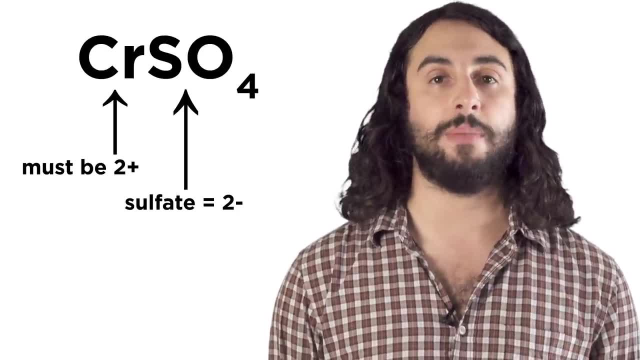 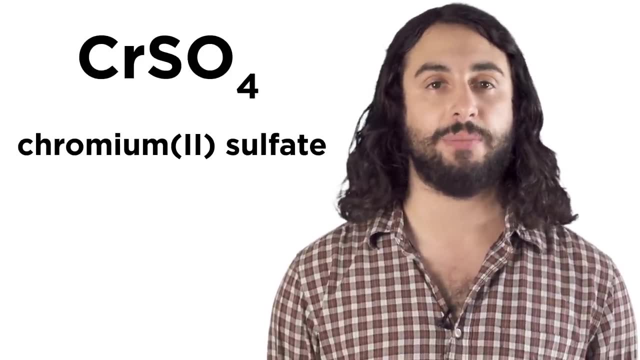 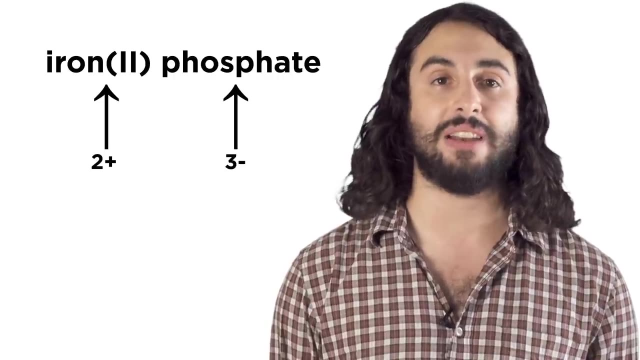 Here the sulfate is 2-, so we know the chromium atom must be 2+, So this is chromium sulfate. We can also go from a name to a formula unit. If we have the name iron phosphate, we know that we have iron atoms that are 2+ and phosphates that are 3-.